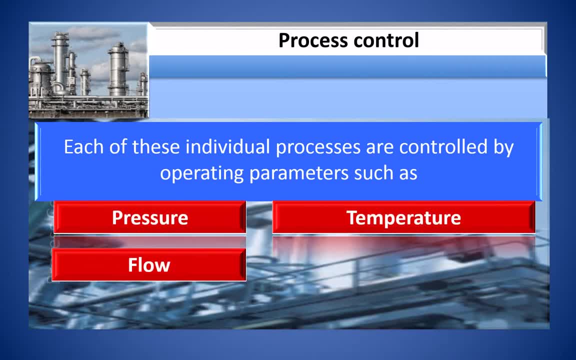 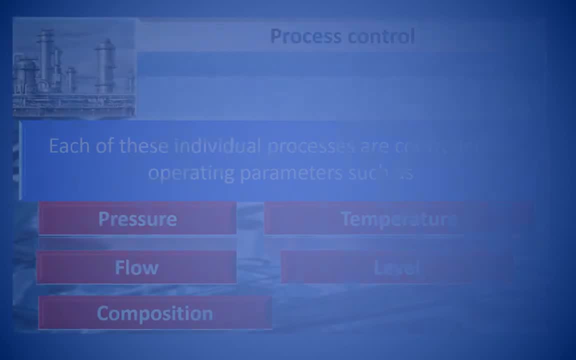 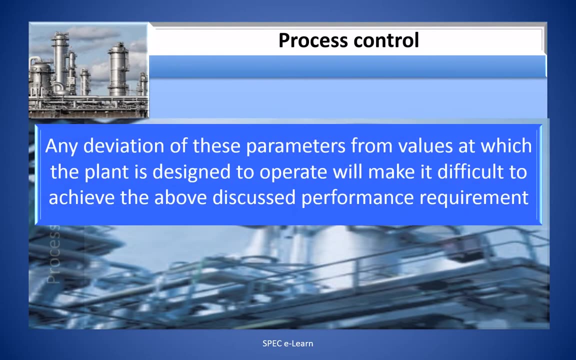 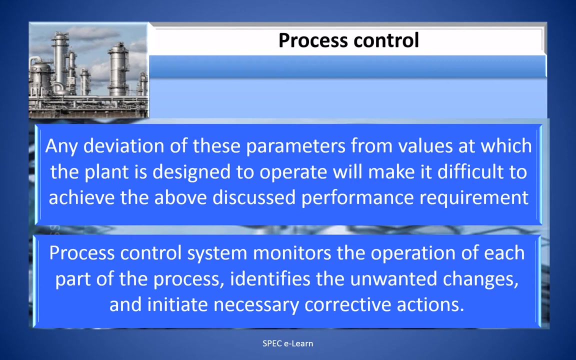 as pressure, temperature, flow level, composition, etc. Any deviation of these parameters from values at which the plant is designed to operate will make it difficult to achieve above discussed performance requirement. Process control system monitors the operation of each part of the process, identifies the unwanted changes and initiate necessary 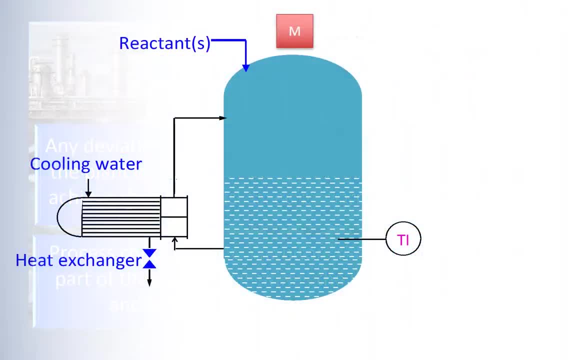 corrective action. This figure illustrates a homogeneous batch reactor in which an exothermic reaction is taking place. The temperature rises during the reaction. The temperature is to be controlled during the reaction. To control the temperature, the contents of the reactor is withdrawn from the reactor and circulated through. 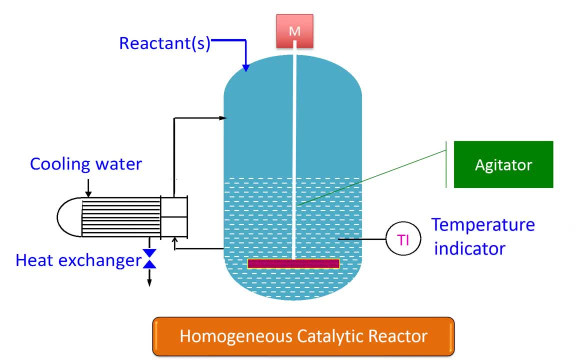 an external heat exchanger, A temperature indicator, Ti, measures and records the temperature of the reactor. Assume you have two systems, one with manual control and another with automatic control How the temperature of the reactor system varies with the time. with these two different control systems, 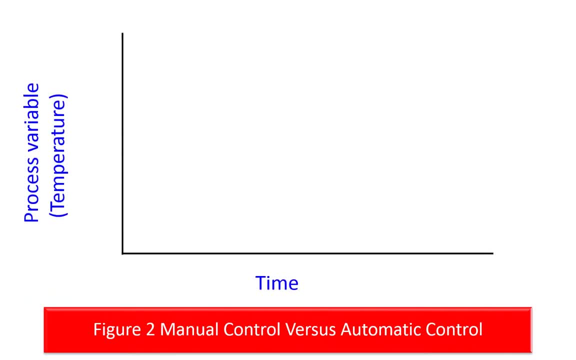 The variation of the reactor temperature is illustrated in this figure. This is a plot of operating variable temperature versus strength. Let us assume that the reactor temperature is to be maintained at 80 degree centigrade In the manual control. the cooling water to the cooler is regulated manually by the operator. 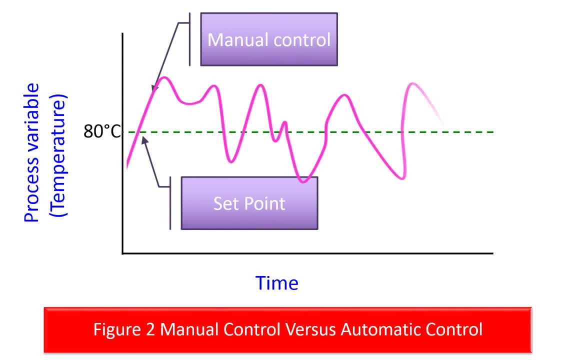 to control the temperature. hence it swings widely. In the automatic control system, the cooling water flow to the cooler will be controlled automatically with no operator intervention. hence it has much less variation. The temperature is maintained within a narrow range. This is the benefit of automatic control. 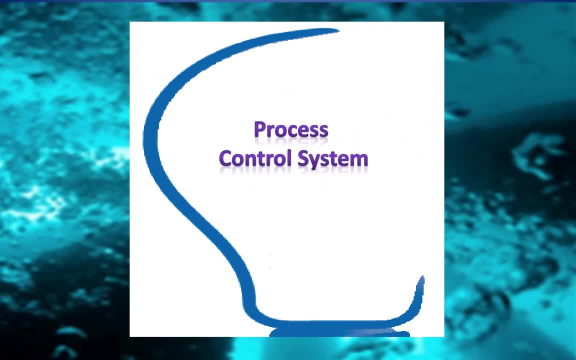 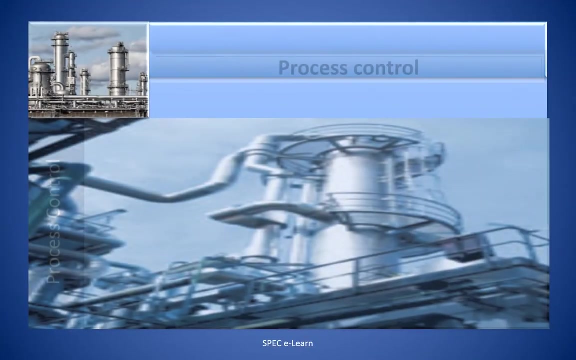 Process control system. How does a process control system work to control the process parameters with a narrow range of the desired operating point? Let us move on to find out. We are understanding what is process control system, who developed them and how it works. 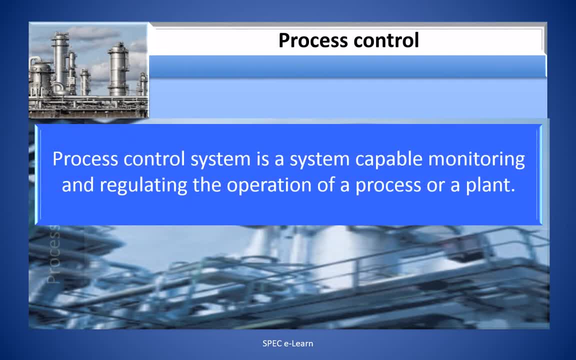 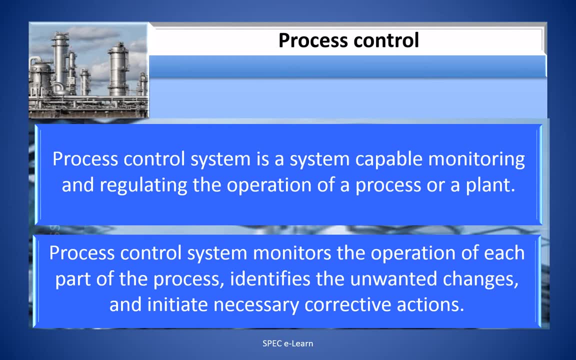 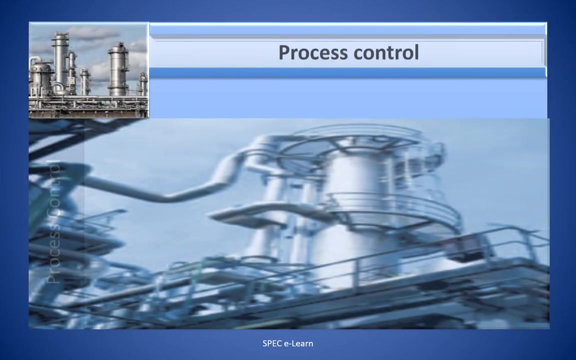 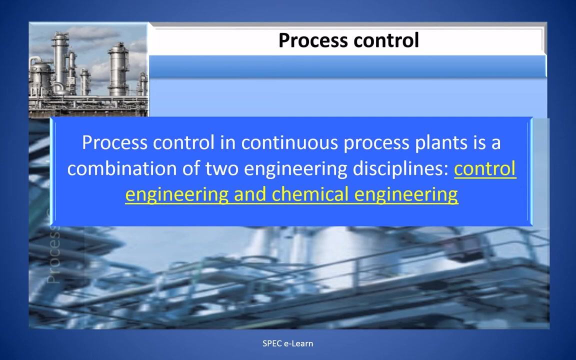 Process control system is a system capable of monitoring and regulating the operation of a process or a plant. Process control system monitors the operation of each part of the process. It identifies the unwanted changes and initiates necessary corrective actions. Process control in a continuous process plant is a combination of two engineering disciplines. 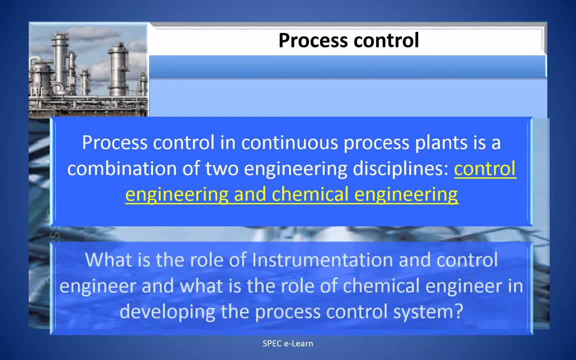 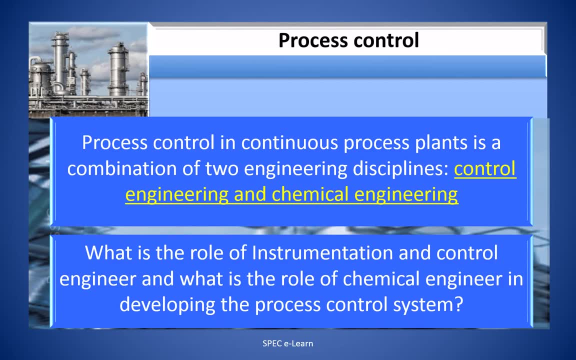 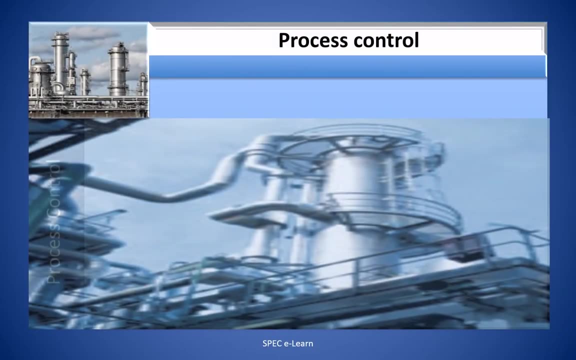 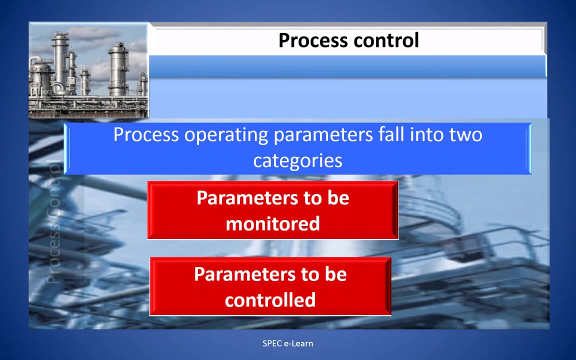 control engineering and chemical engineering. What is the role of instrumentation and control engineer and what is the role of chemical engineer in developing a process control system? Process parameters fall into two categories: parameters to be monitored and parameters to be controlled. All the operating parameters measured need not be controlled. 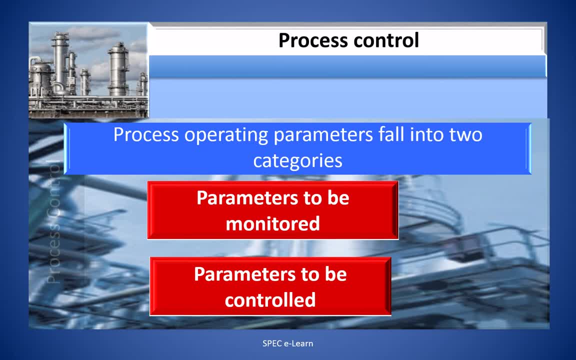 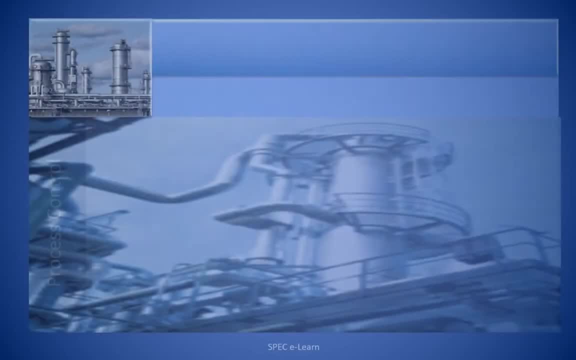 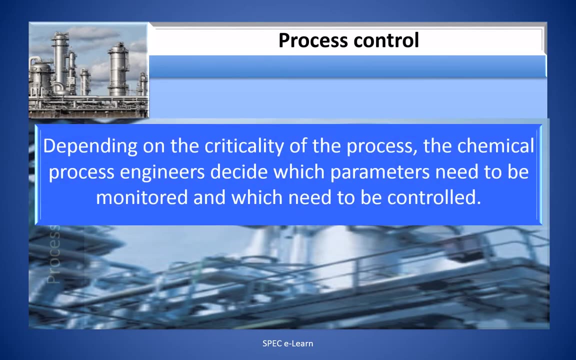 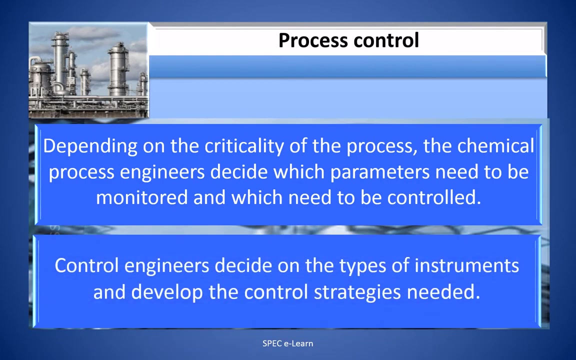 Some are required for monitoring the process conditions and others are key parameters which need to be controlled. What is process control system and what is process control system? Depending on the criticality of the process, chemical process engineers decide which parameters need to be monitored and which need to be controlled. 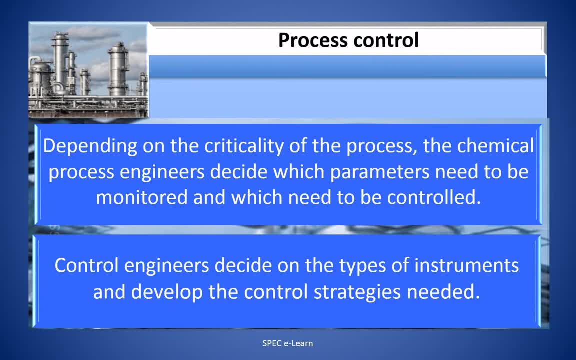 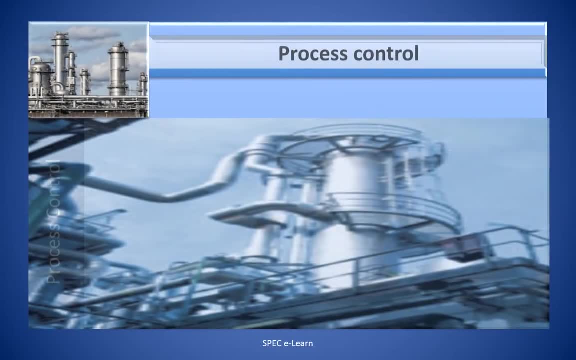 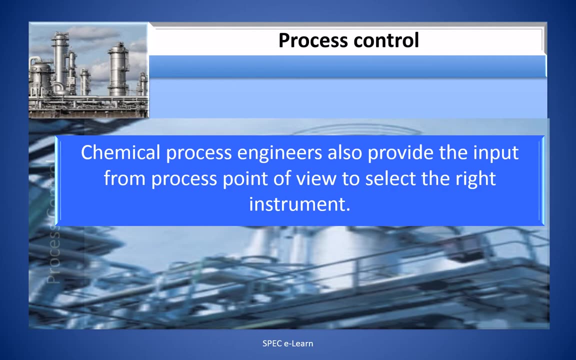 Control engineers decide on the type of instruments and develop the control strategies needed. What is Africa's most useful component? Africa's most useful component is the chemical process. What is Africa's most useful component? provide the input from the process point of view to select the right instrument. 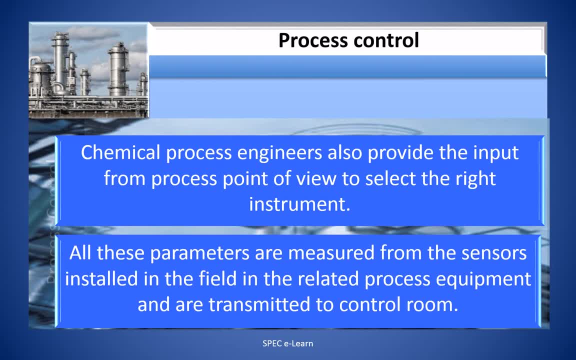 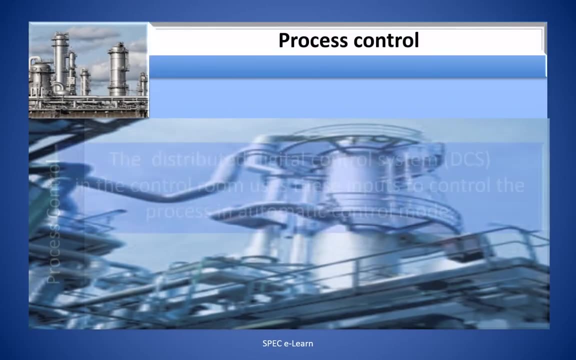 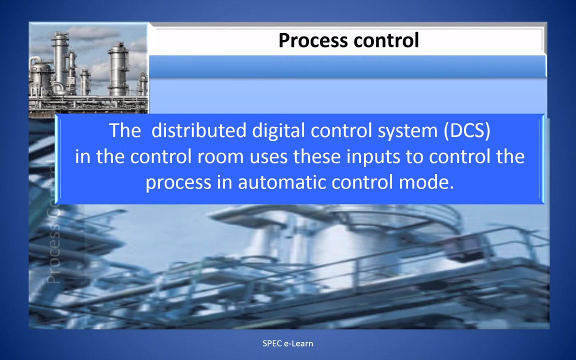 All these parameters are measured from the sensors installed in the field in the related process equipment and transmitted to the control room. The Distributed Digital Control System in the control room uses these inputs to control the process in automatic control mode. Some process plants may also have other. 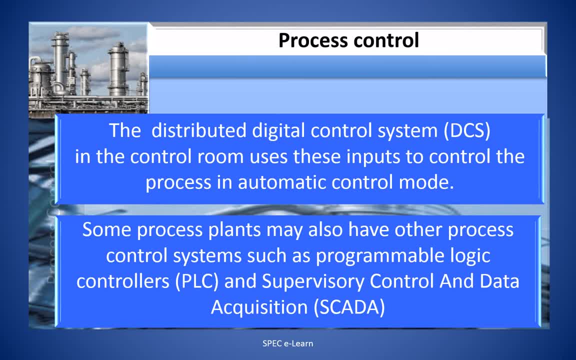 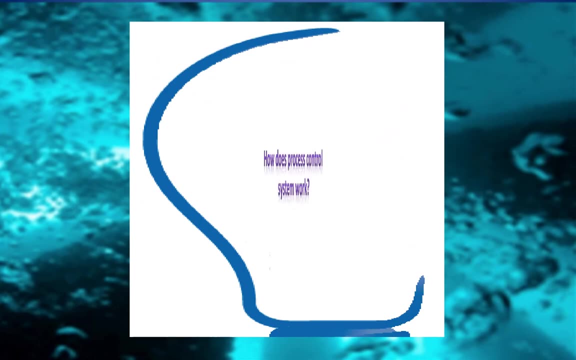 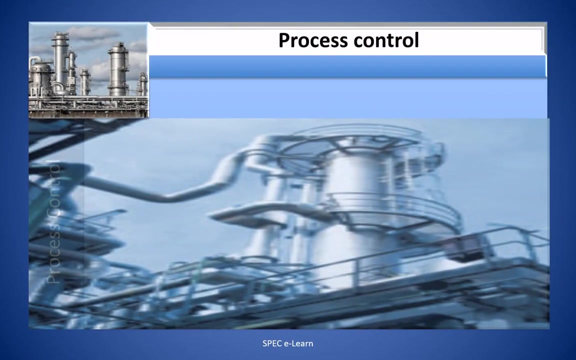 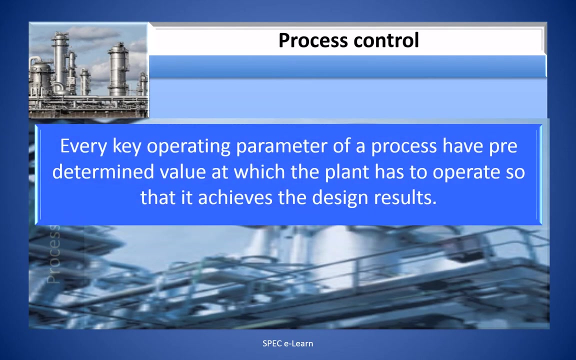 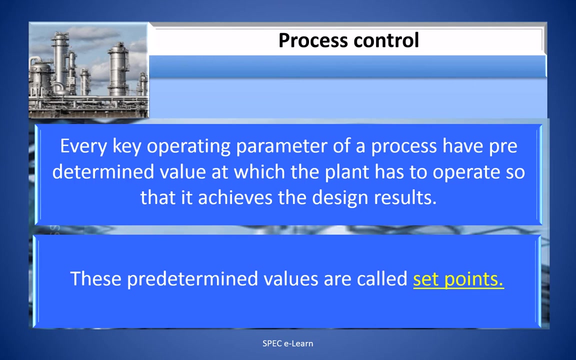 process control systems, such as Programmable Logic Controllers and Supervisory Control and Data Acquisition System. How does the Process Control System work? Every key operating parameter of a process has a pre-determined value at which the plant has to operate so that it achieves the desired results. These pre-determined values are called set points. 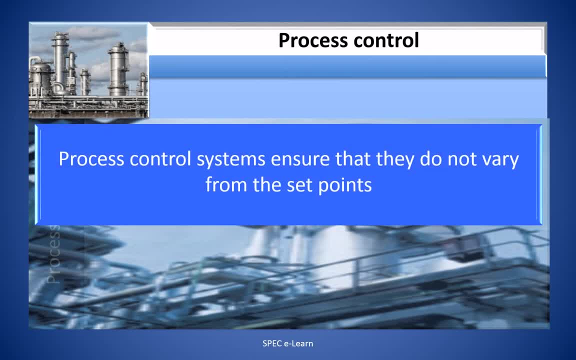 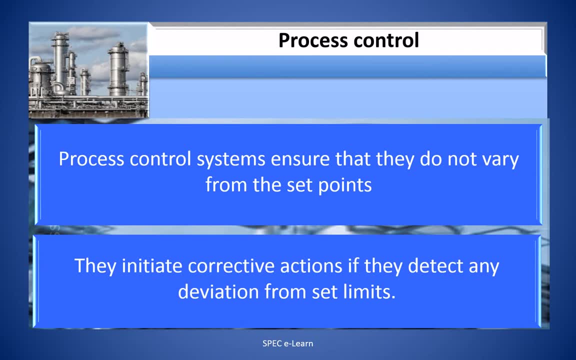 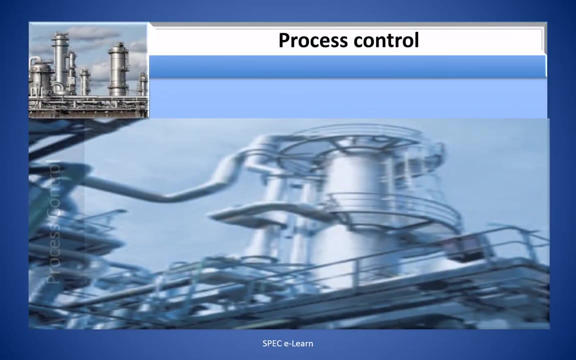 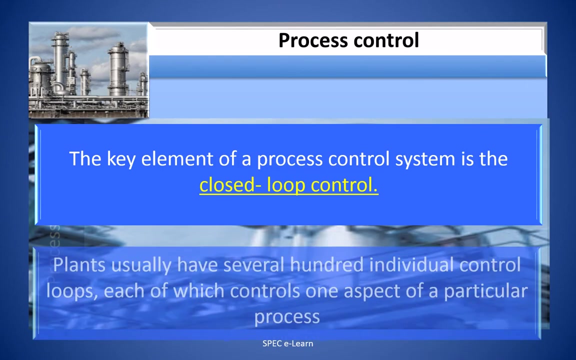 Process Control Systems ensure that they do not vary from the set points. They initiate corrective actions if they detect any deviation from the set limits. The key element of a Process Control System is the Closed Loop. Control Plants usually have several hundred individual control loops, each of which controls one aspect of a particular process. 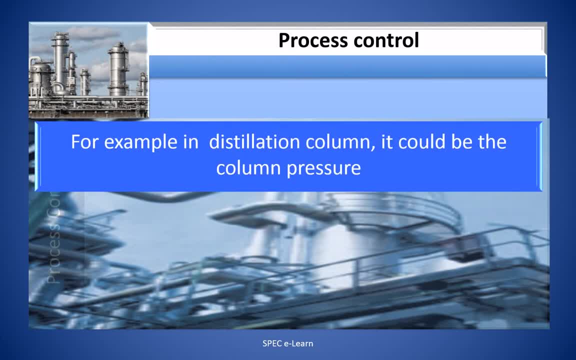 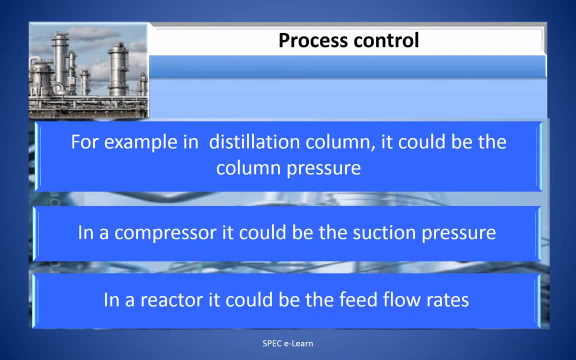 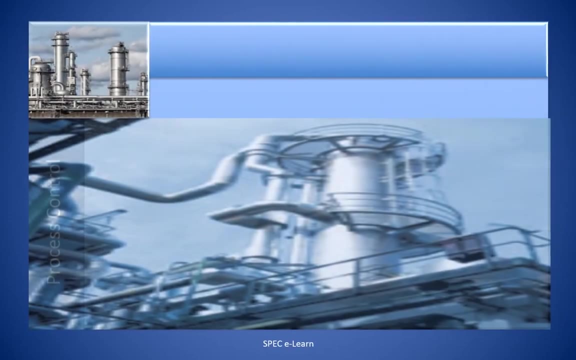 For example, in the distillation column it could be the column pressure. In a compressor, it could be the suction pressure. In the reactor, it could be the feed flow rate. The function of the control loop is to ensure that a particular parameter is maintained at 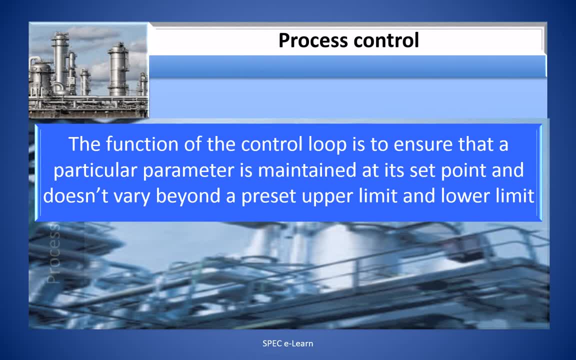 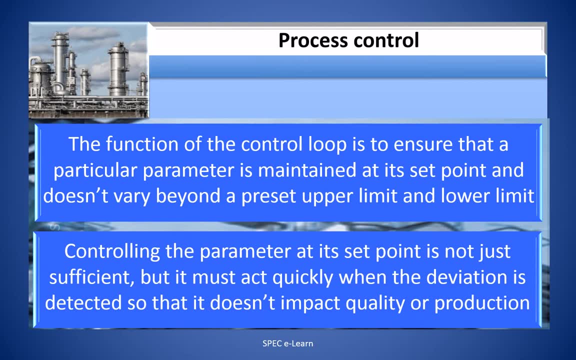 its set point and does not vary beyond the set point. The process function is to transmit the pressure to the control room from the Compressor. This is a point to be a preset: upper limit and lower limit. Controlling the parameter at its set point is not just sufficient, but it must act quickly when the deviation is. 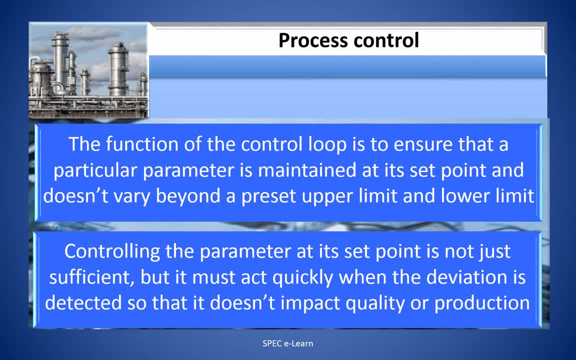 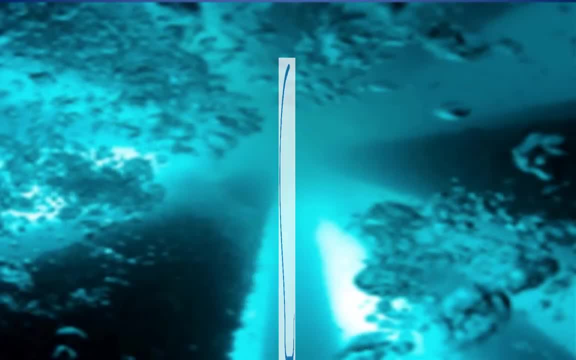 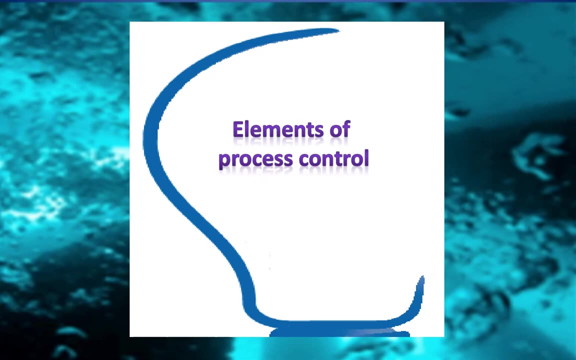 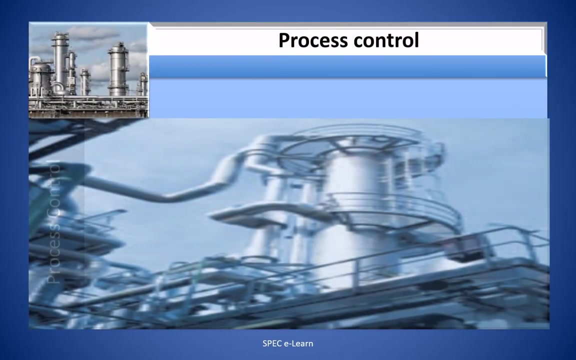 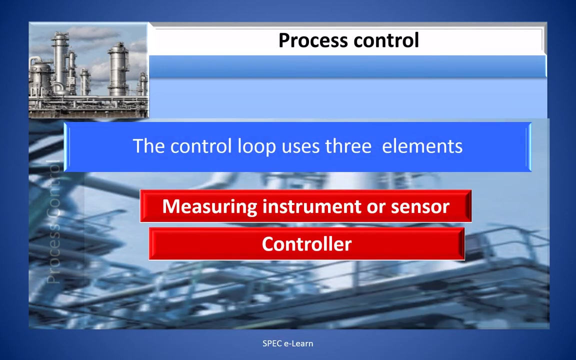 detected so that it does not impact quality or the production. Having understood how the control system works, let us now move on to the elements of process control. The control loop uses three elements: machine element or sensor controller and final control element or the control valve. How do the three elements work? 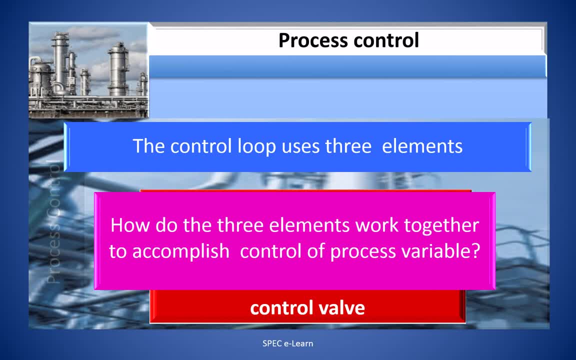 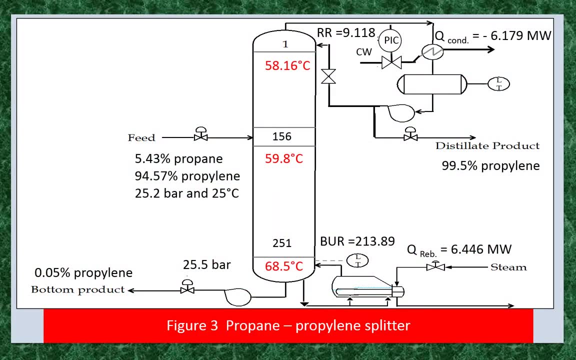 together To accomplish the control of process variables. Illustrated in this figure is a distillation column operated by automatic process control system. The column has several key process variables that need to be controlled, For example, feed rate, reflux, flow rate, column pressure, reflux, drum level, etc. 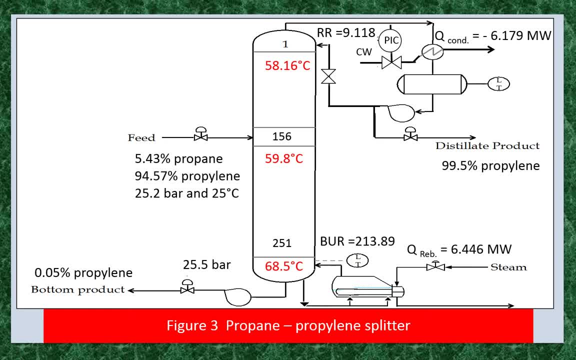 Let us consider one of the key variables, the pressure. for our understanding of process control system, This is done by a pressure controller. The process control loop for pressure control is called PAC, Pressure Indicator Comptroller. The PAC controls the pressure at around the set point. The set point is the desired value. 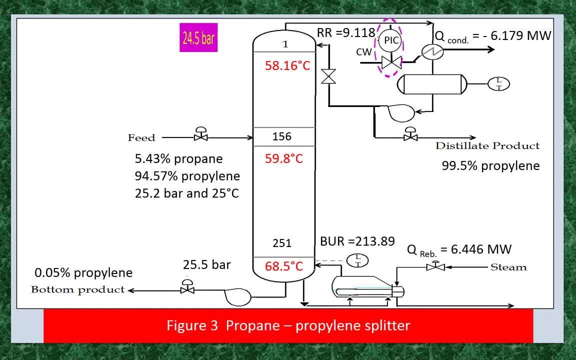 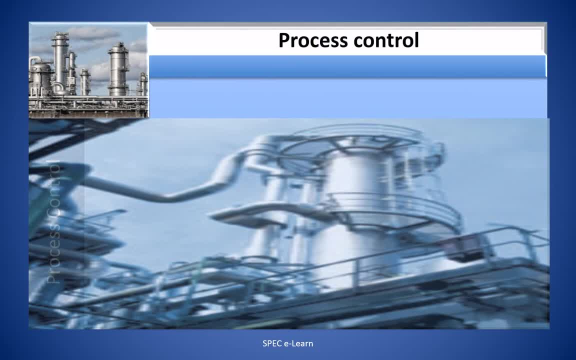 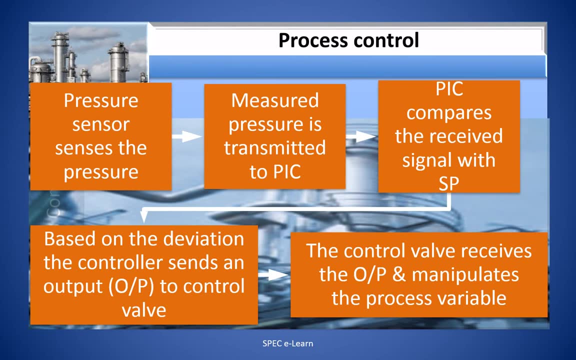 of the pressure at which the column is designed to operate. Now let us look at the exercise. The pressure sensor senses the pressure. The measured variable is transmitted to the PAC, The AC compass, the received signal with the setpoint. Based on this, the outcome of the verder darkness pump morning. the evaluation is the result. 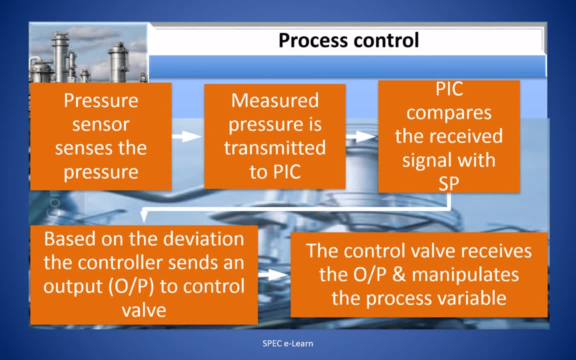 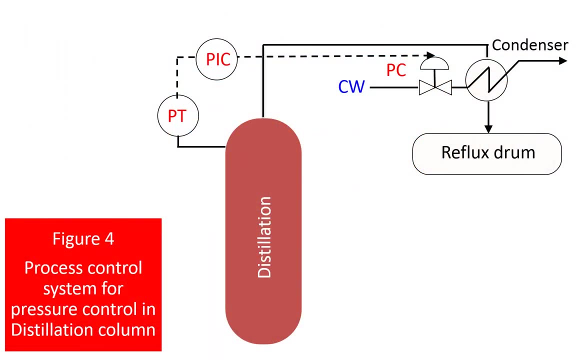 Let us go deeper the deviation. the controller sends an output to the control valve. The control valve receives the output and manipulates the process variable. The elements of process control for the pressure control system of the distillation column is shown in this figure. 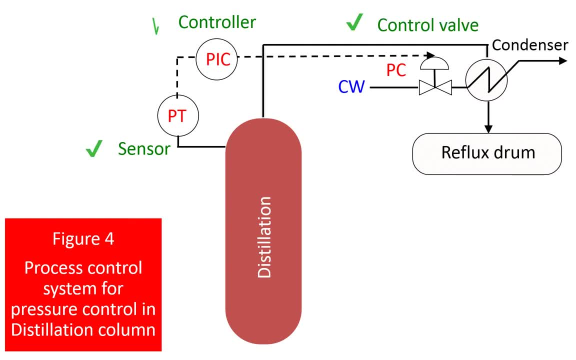 In one example of distillation column, the set point of the pressure controller is 24.5 bar. If the measured variable is 24 bar, it is below the set point and the controller sends a signal to the final control element to reduce the cooling water flow to the condenser. 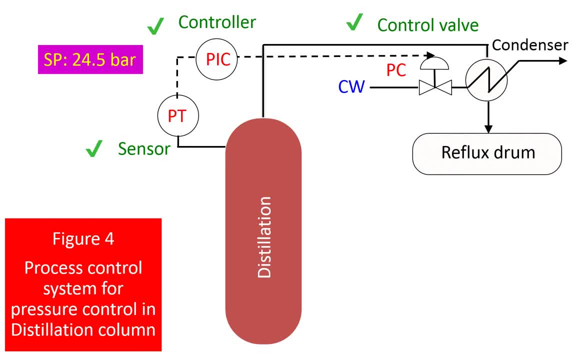 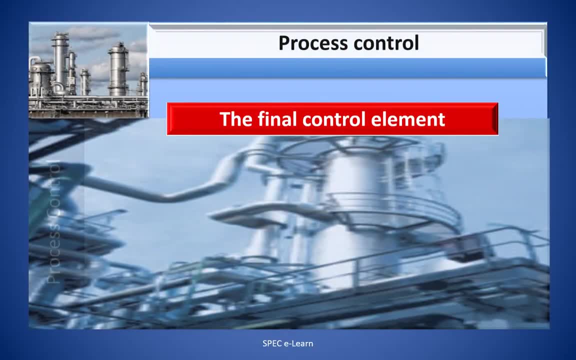 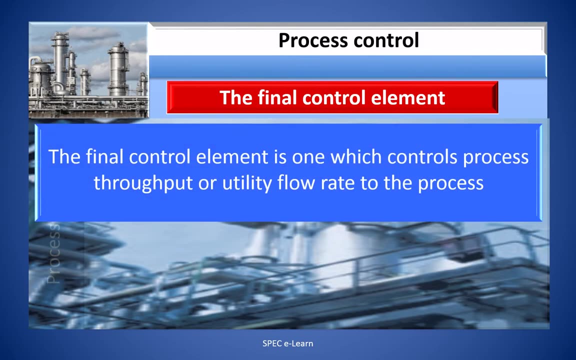 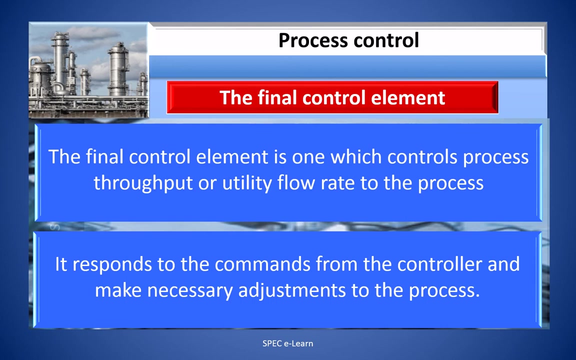 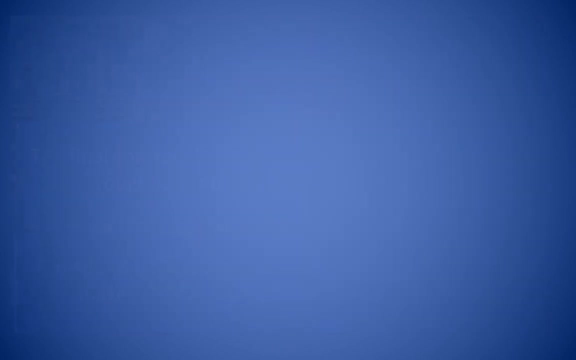 so that the pressure is increased back to 24.5 bar. What is the final control element? The final control element is one which controls the process throughput or utility flow rate to the process. It responds to the commands from the controller and makes necessary adjustments. 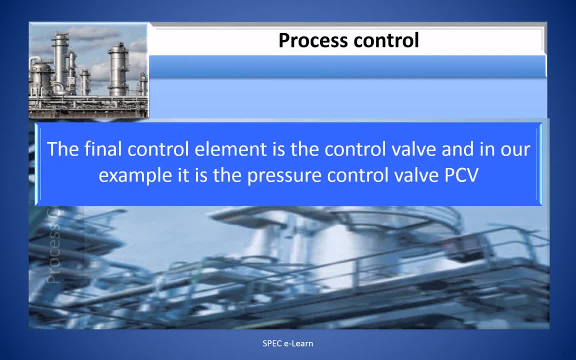 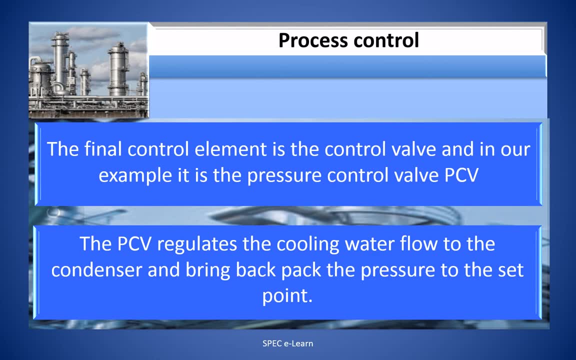 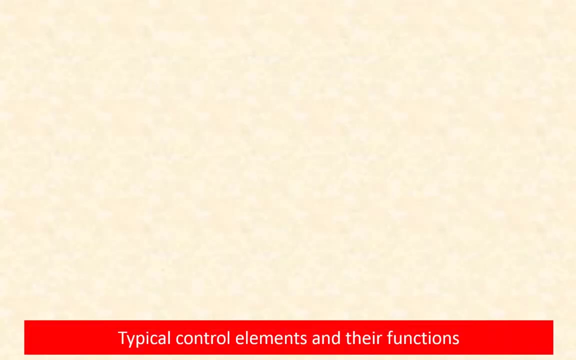 The final control element is the control valve. In your example it is a pressure control valve, PCV. The PCV regulates the cooling water flow to the condenser and bring back the pressure to the reset point. So what are the elements of process control? 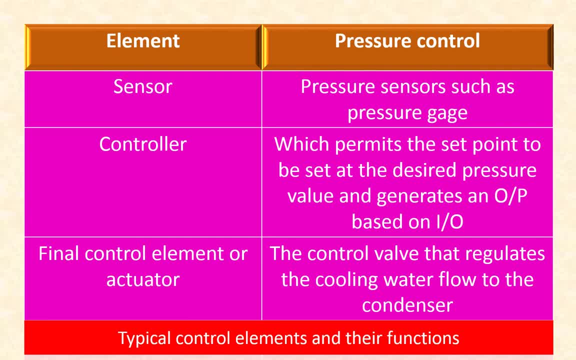 It is explained here with an example of pressure control system for the distillation column Pressure sensor. the pressure sensor, such as the pressure gauge Controller, which permits the set point to be set at the desired pressure value and generates an output based on the input. 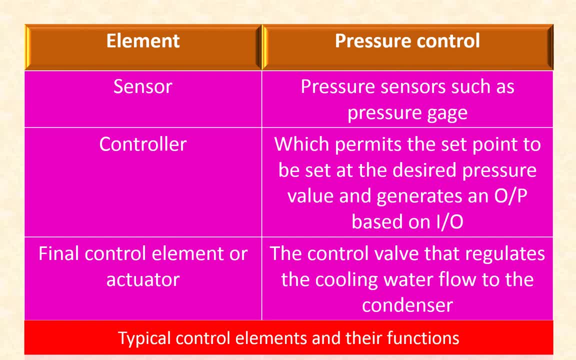 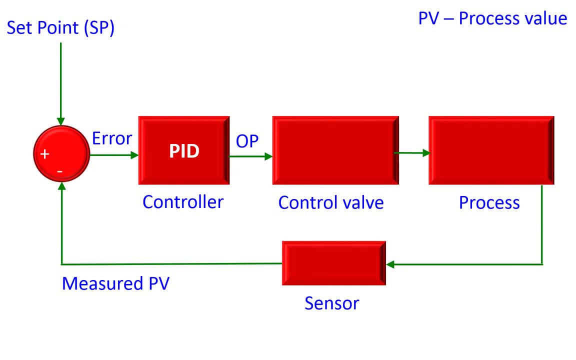 Final control element, or the actuator, the control valve that regulates the cooling water flow to the condenser. The block diagram showing the blocks of a control system is shown in this figure. In most cases, the error term is used to calculate the controller output. 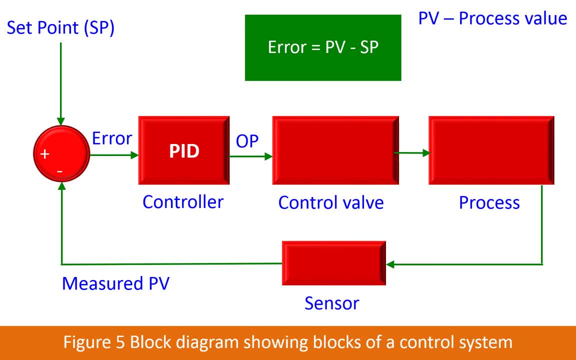 The error is equal to PV minus SP, where PV is the process value and SP is the set point. The variable that the control valve regulates is called the manipulated variable. This could be the feed flow or reflux flow in the case of a distillation column or cooling. 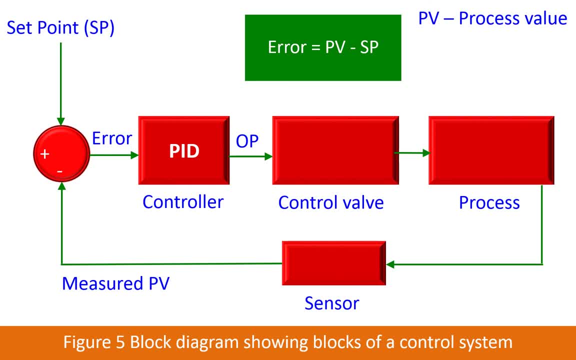 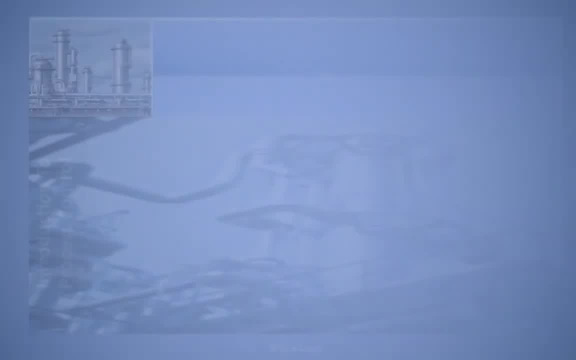 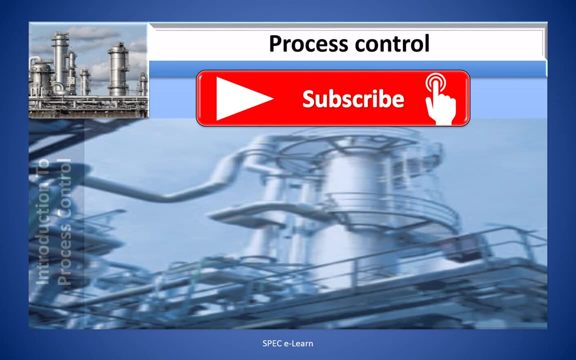 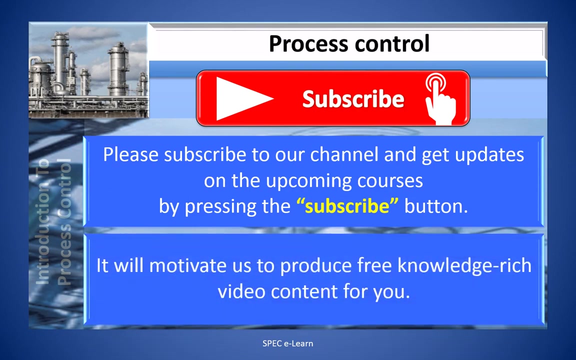 water or steam or any other iterative flow rate which has an effect on the production process variable. Please subscribe to our channel and get updates on the upcoming courses by pressing the subscribe button. It will motivate us to produce free knowledge, rich video content for you.